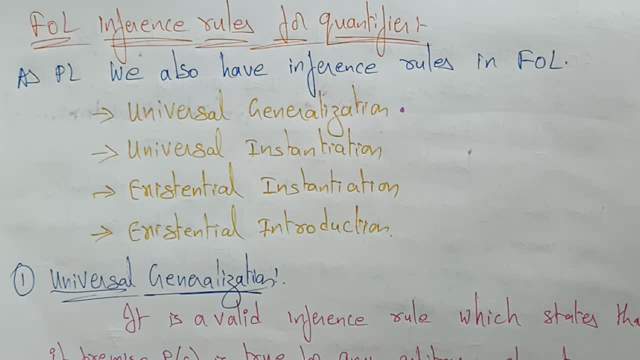 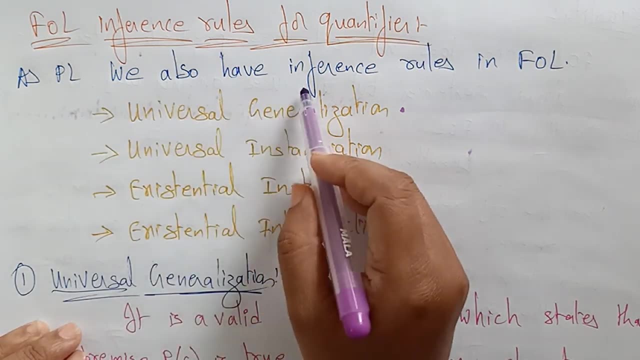 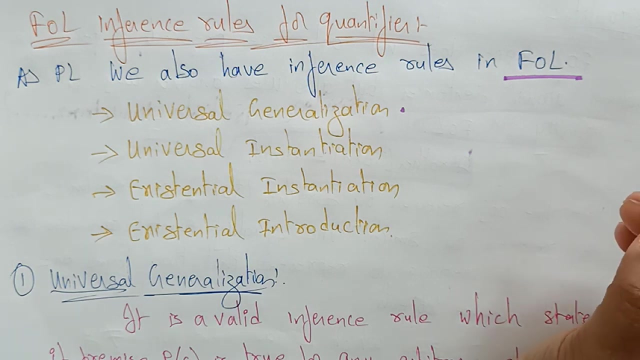 explain you the inferences rules for the quantifiers in the first order logic. So as propositional logic, we also have the inference rules in first order logic. So not only for the propositional logic in the first order logic, also some inference rules are there. 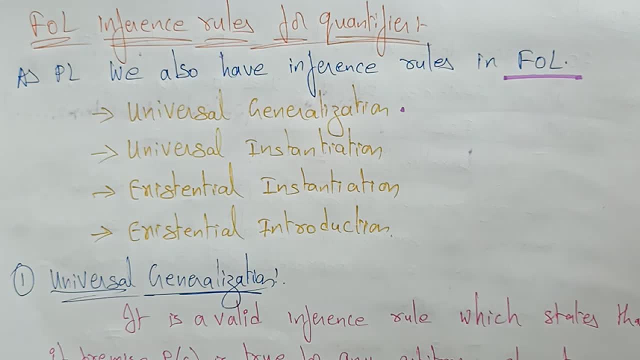 So in the previous video I explained about the inferences for the propositional logic also. If you want, you just go through that video and here also in the same way, the first order logic is also having some inference rules. So what are those? Those are universal generalization. 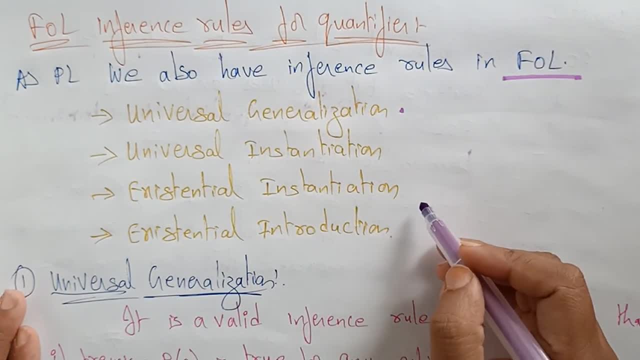 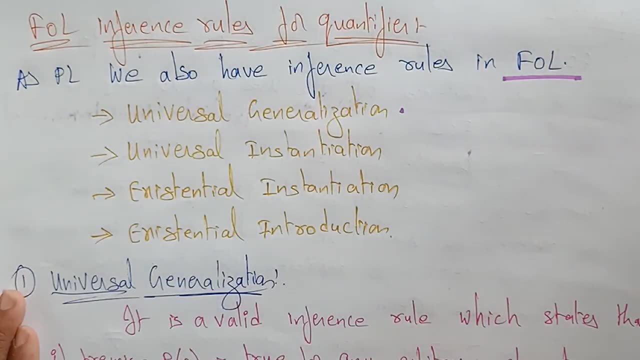 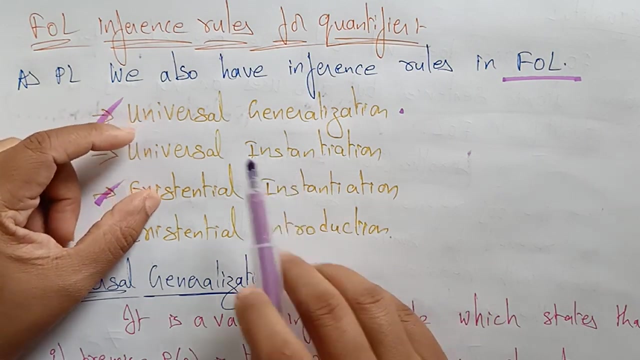 universal instantiation, existential instantiation and existential introduction. Actually, universal and existential are the two quantifiers that we know. that right, These two are the quantifiers. universal and existential are the quantifiers. So the inference rules for this is universal generalization, universal instantiation, In the same way existential instantiation. 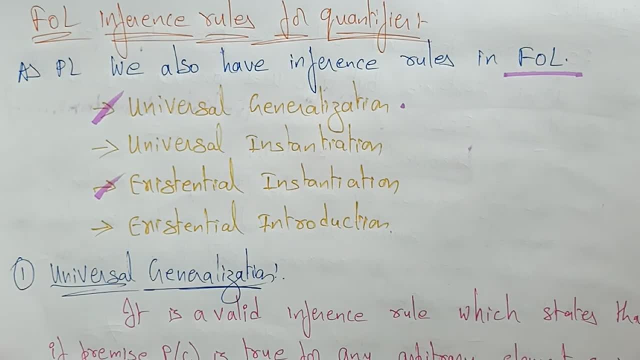 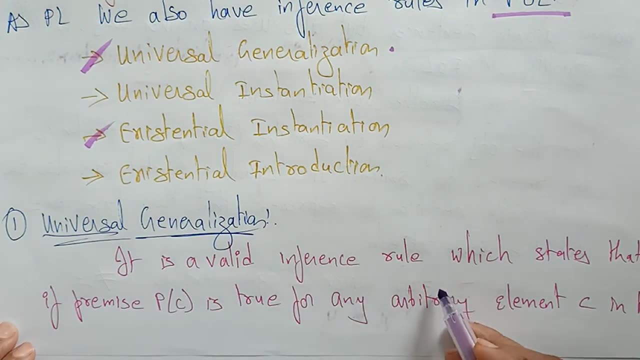 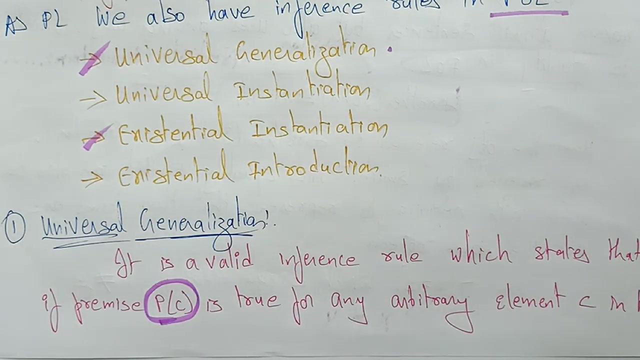 and existential introduction. Let's see one by one. what is this universal generalization? Universal generalization, it is a valid inference rule which statement that if premises P of C is true. Let me tell you the definition first. Later I will explain with an example. Don't be confused. 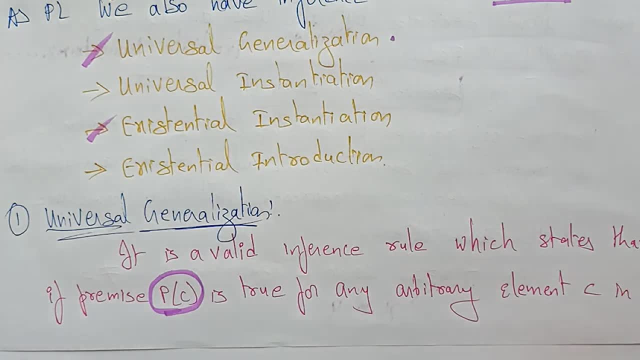 Okay, if you didn't understand the definition, don't bother about it. If you see the example, then you can clearly understand what is this universal generalization? So the universal generalization is a valid inference rule. Why I am saying this is a valid inference rule. 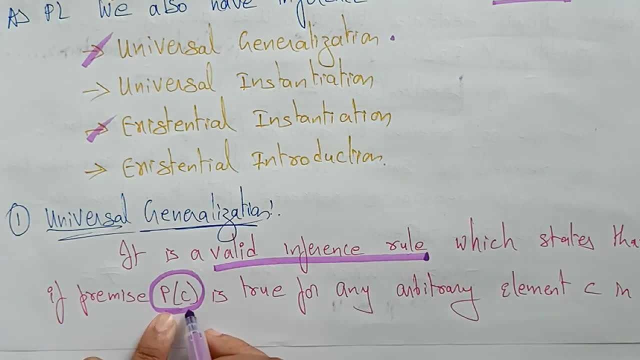 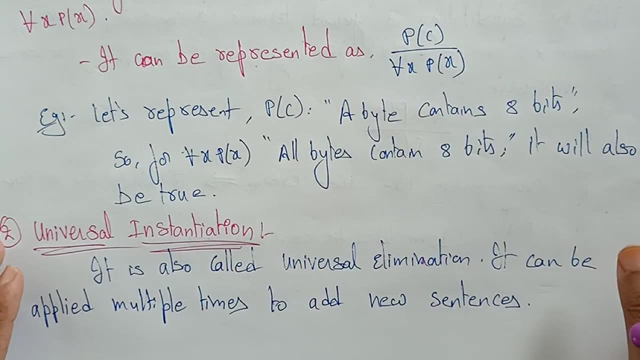 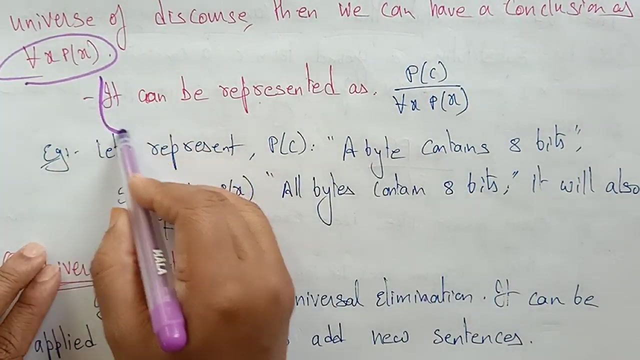 Because which statements that if premises P of C is true for any arbitrary element C in the universe of this curse, Then we can have a conclusion: as for all x, P of x. So this, the universal generalization, can be represented as P of C. This is a premises P. 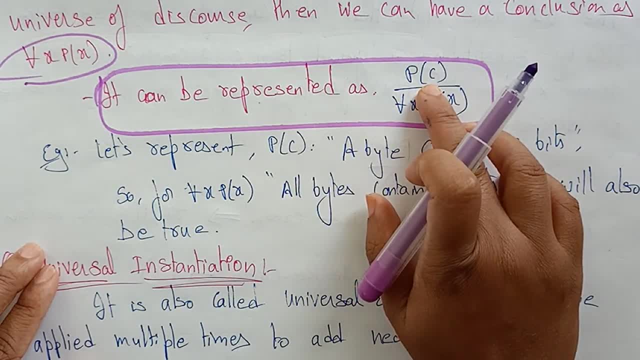 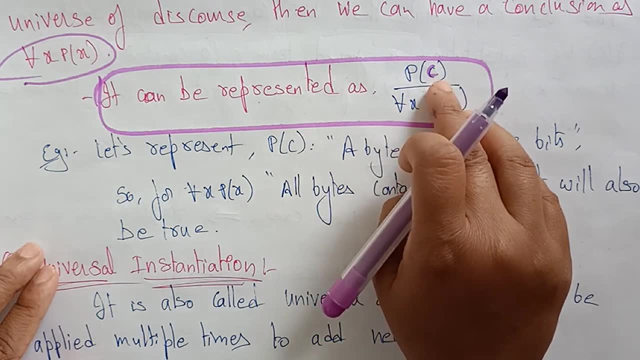 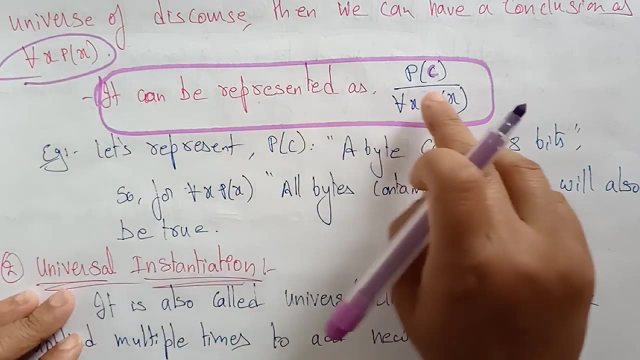 of C is true for any arbitrary of element C. So here this is an element Okay, which is the premises of C is true, But the universe of discourse, that we can have a conclusion like for all x, P of x, So P of C by for all x, P of x. I will explain with an example. 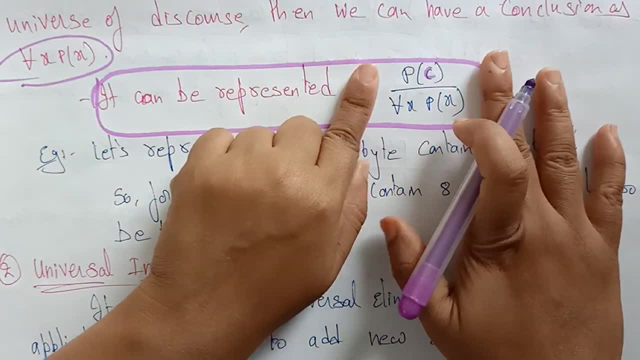 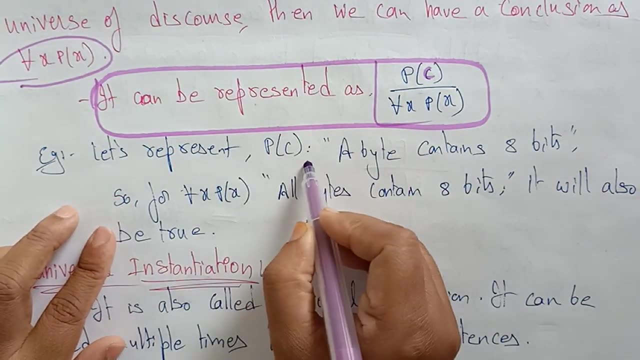 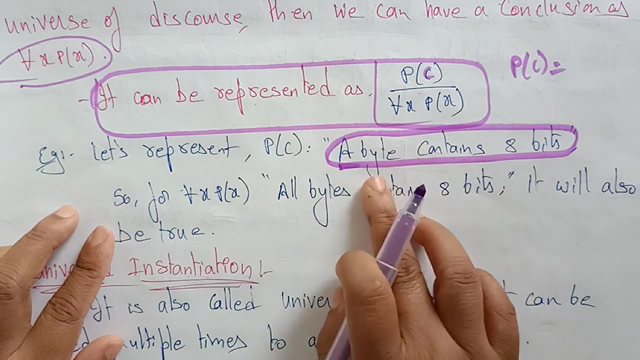 Don't confuse. but you have to remember that the universal generalization can be represented like this: P of C by for all, x, P of x. So let's represent P of C. Let me take a statement: A, P of C. I am taking a statement like a byte contains 8 bits. A byte contains 8 bits, So this is: 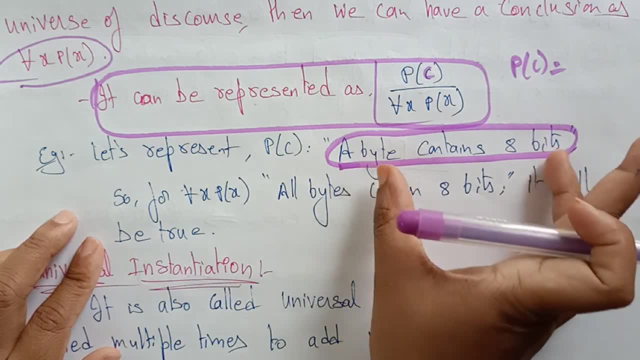 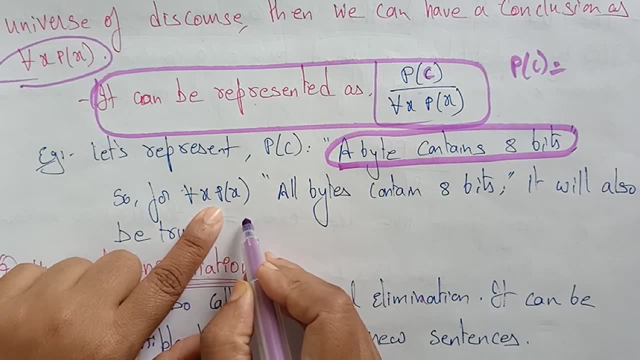 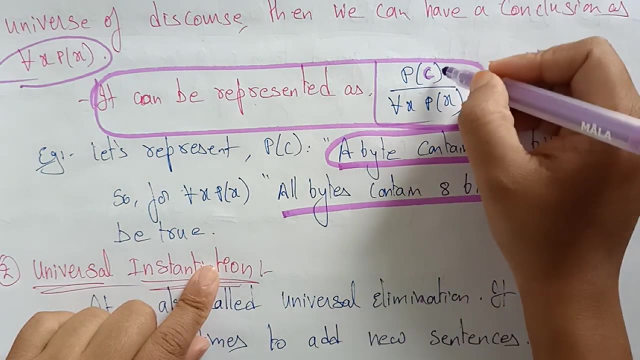 a predicate, Okay, a statement, with an arbitrary element C. A byte contains 8 bits, So for all x, P of x is nothing, but all bytes contain 8 bits. It will also be true, Is it Suppose, if a particular byte contains 8 bit, means then all bytes. 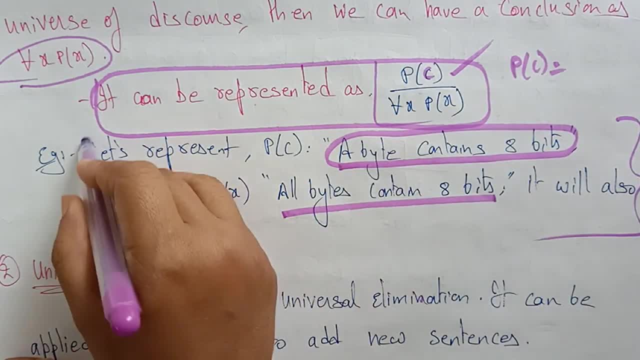 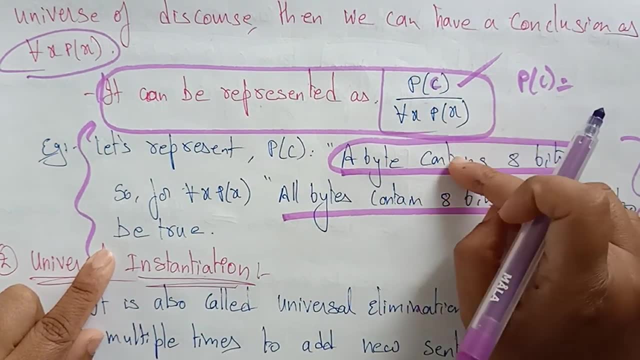 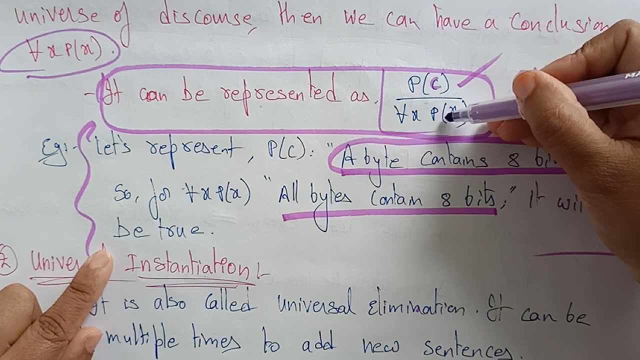 all bytes contains 8 bits. So this is universal generalization. So when it is true means obviously this is also true. So this statement I had represented in this universal generalization: A byte contains 8 bit. That means for all bytes. all bytes contains 8 bits, All bytes contains 8. 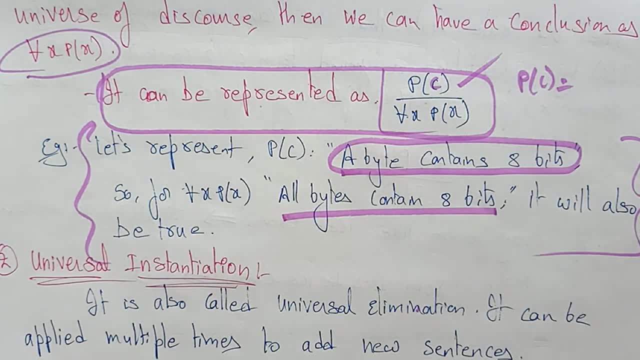 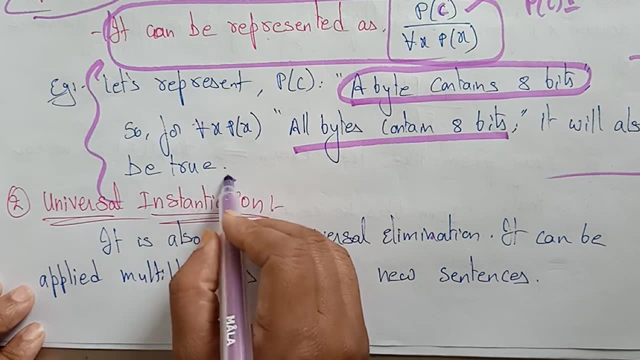 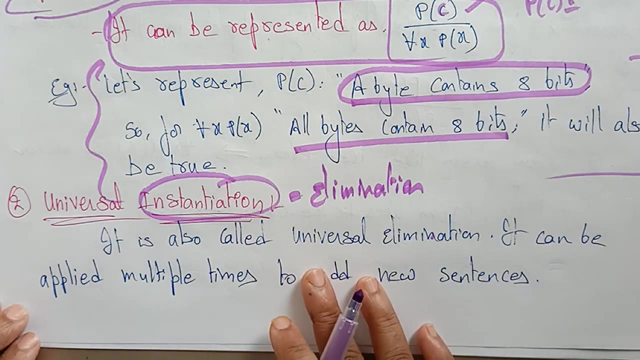 bits. Is it clear? Now let's see the universal instantiation. It is also called universal elimination. The instantiation- you also call it as elimination, So it is also called universal elimination. It can be applied multiple times to add a new sentence. 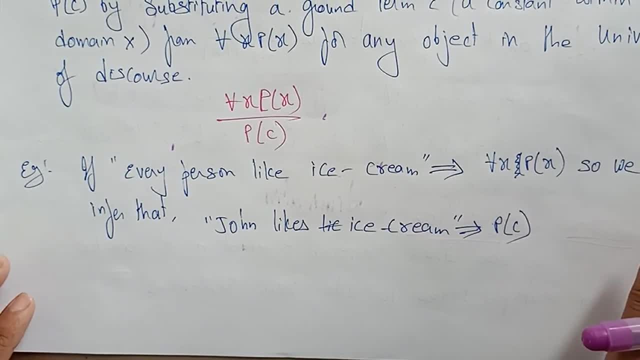 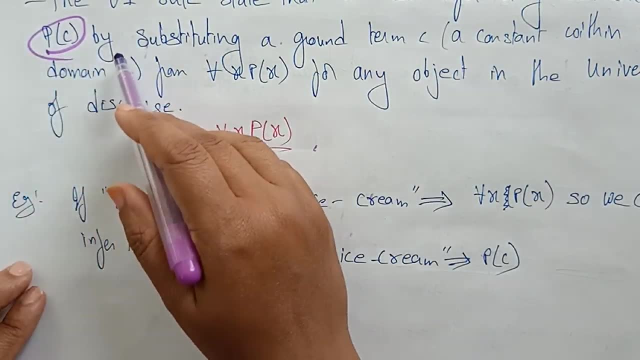 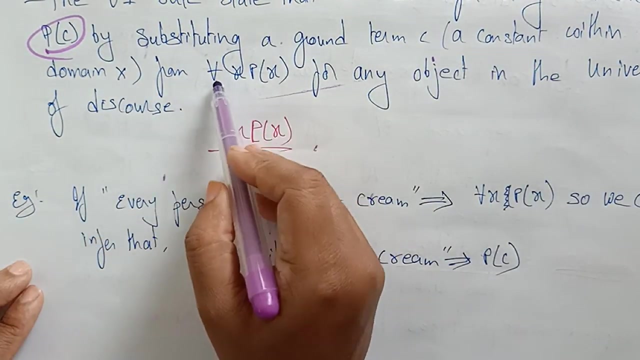 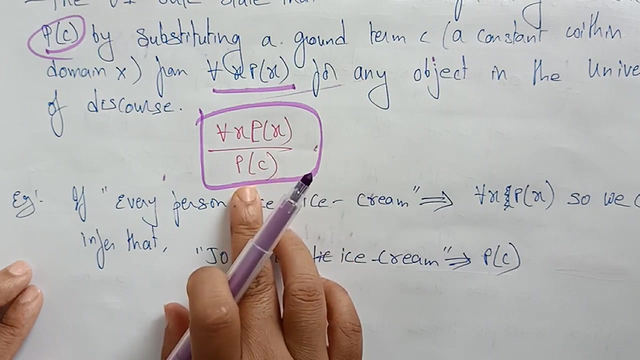 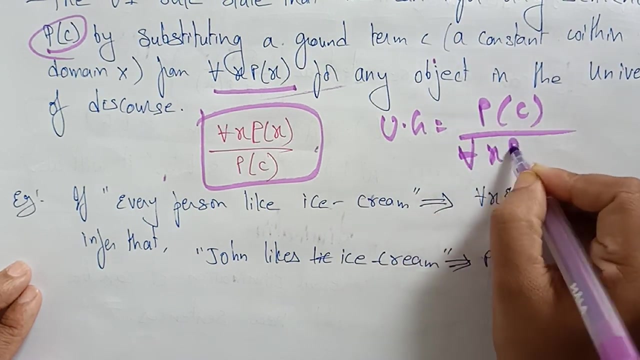 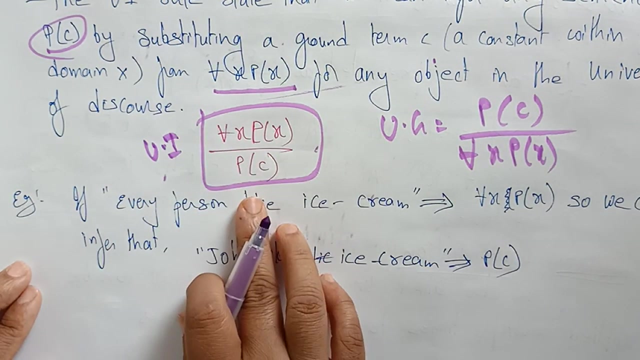 Let's see here: The universal instantiation rule states that we can infer any sentence that is a P of C, that is a premises P of C. See here: The universal instantiation shows that for all X, P of X. So that is the universal generalization and this is the universal instantiation. 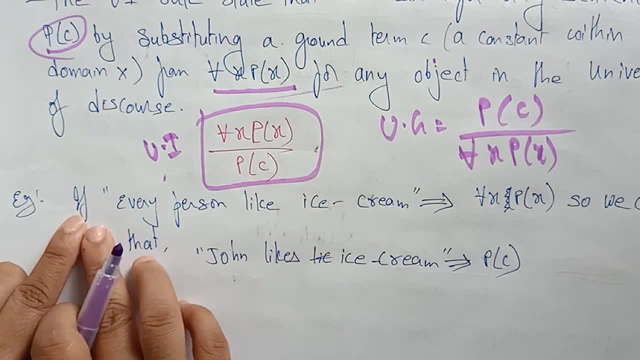 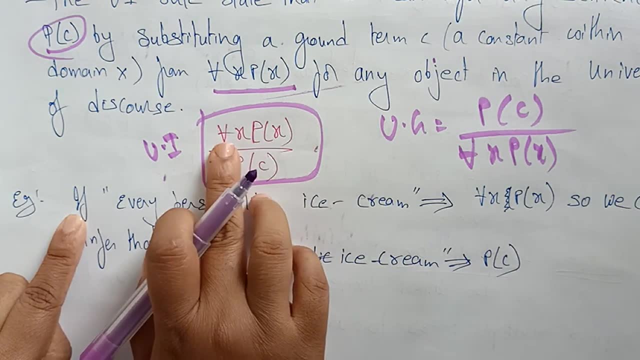 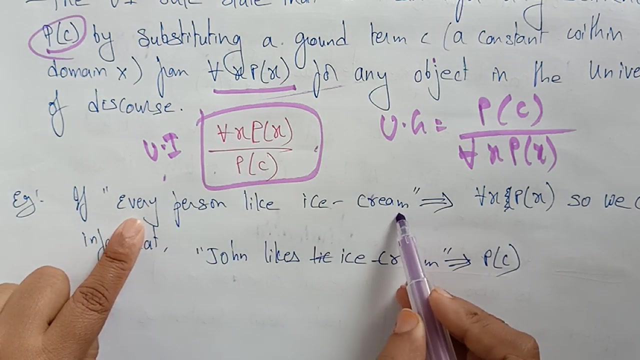 for all X, P of X by P of C. So see here in this example example, every person like ice cream. so this is i'm, uh, actually for all. this symbol is for for all, every and and everything right, so here, every person like ice creams implies this is a representation. 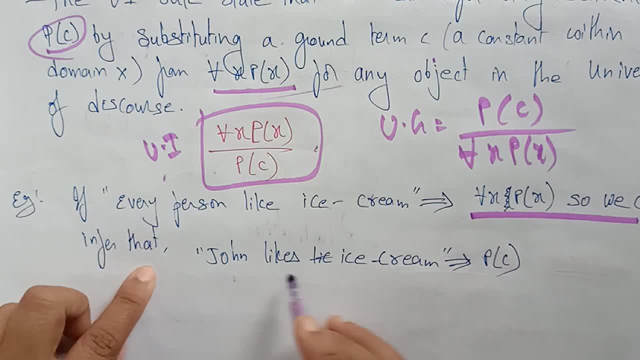 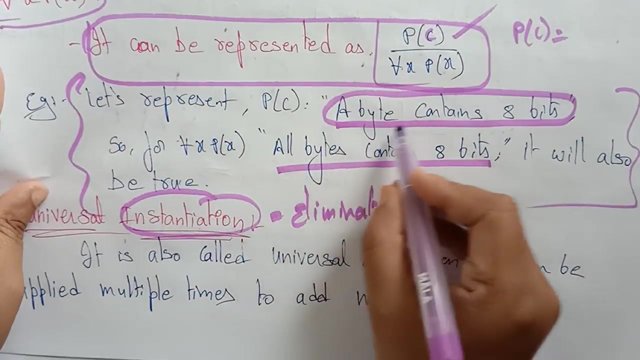 for all x, p of x. so we can infer that john likes ice cream means a particular person where, in this generalization, what i said, a? uh, there i explained that it is a bit okay. so see here, a bite contains eight bits. so this is a p of c, a bite contains eight bits. that means all bites. 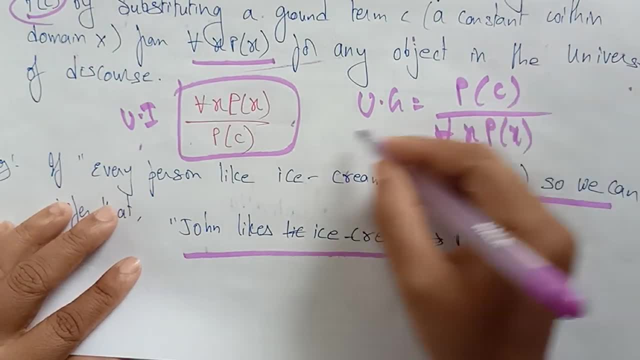 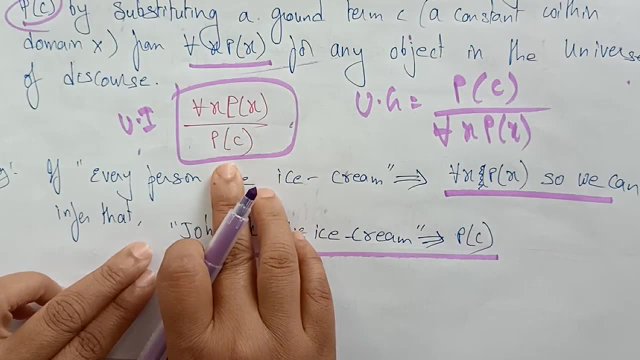 contains eight bits. so in the same way, here every person, every person, likes ice cream. so we can infer that a particular person, that is a john, likes ice cream, a john likes ice cream. you can infer that a particular person that is a john, likes ice cream, a john likes ice cream. 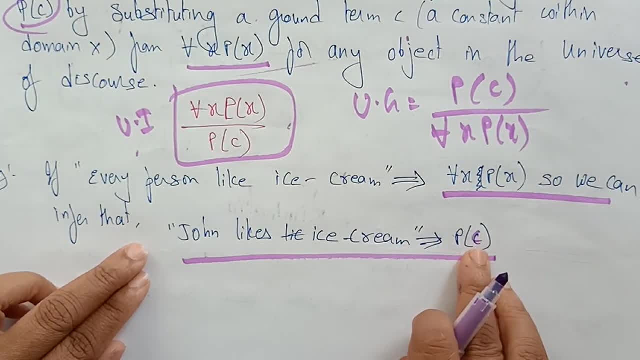 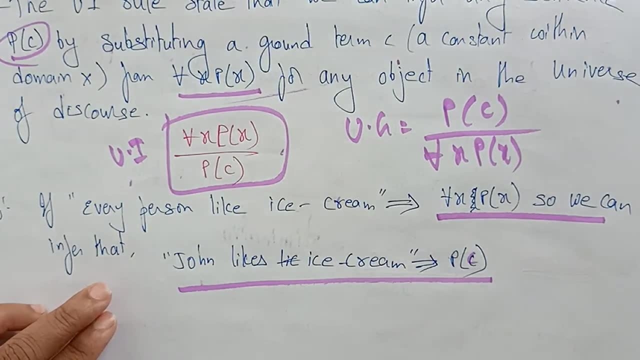 you can infer that a particular person, that is a john, likes ice cream. a john likes ice cream, a particular person, john likes ice cream. so here c is a particular person and here x is every person. x is the every person. this is a universal instantiation. now let's see the another. 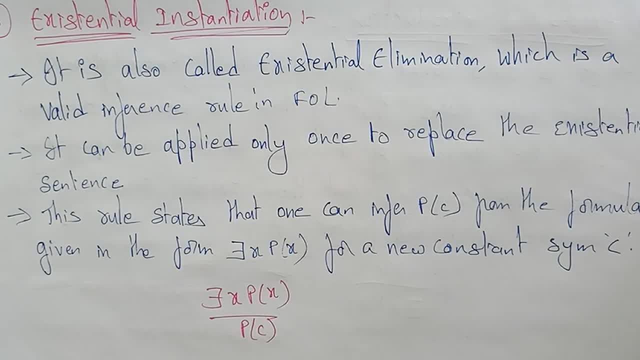 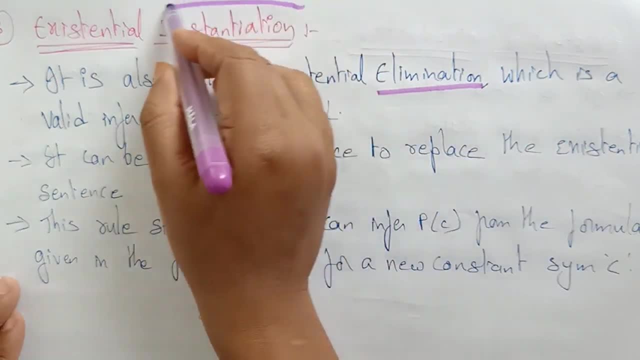 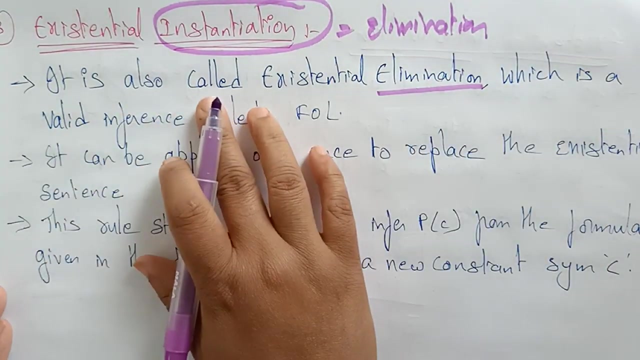 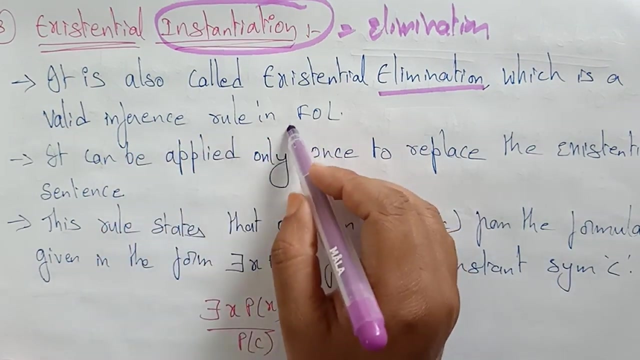 existential instantiation. existential instantiation, so it is also called as elimination. existential elimination- i already said that instantiation you can call it also call it as elimination. so existential instantiation is also called as existential elimination, which is a valid inference rule in the first order logic. it can be applied only once to replace the existential. 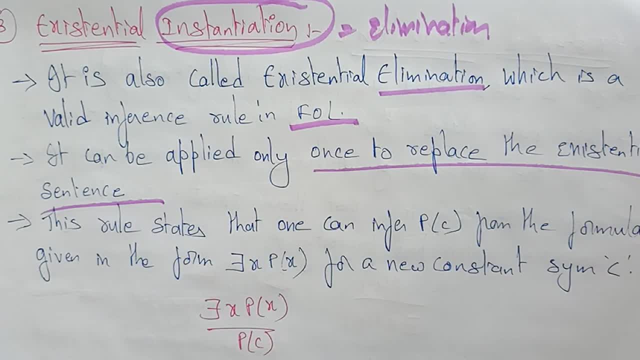 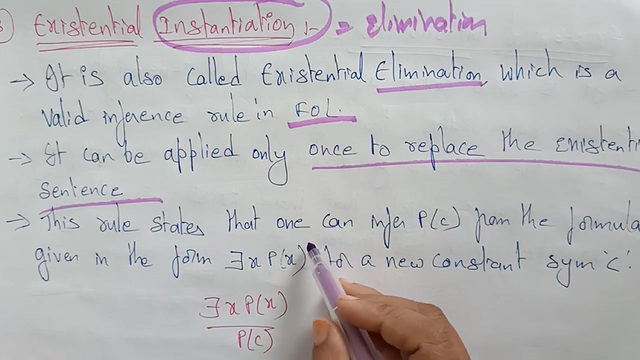 sentence. so here you can only apply once, whereas in this universal instantiation you can apply multiple times to add a new sentence, but in existential only once. you have to apply only once to replace the existential sentence. so you can only apply once to replace the existential existential sentence. So this rule states that one can infer P of C from the rule given in the. 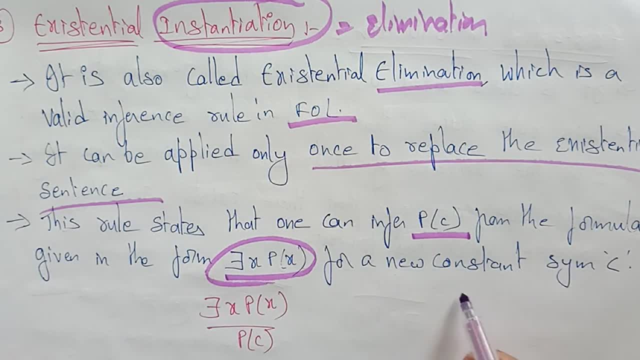 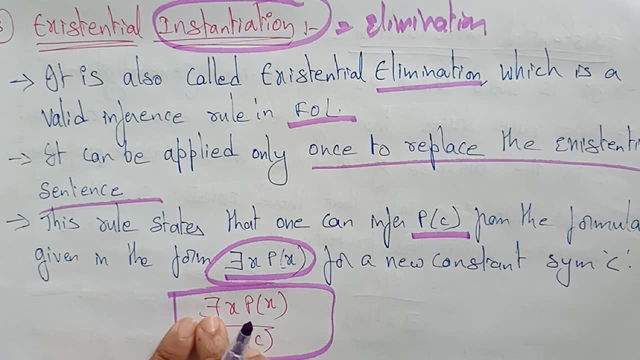 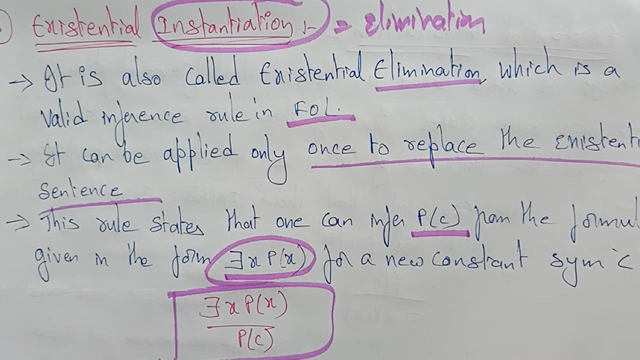 form of: there exist X, P of X for a new constant symbol, C. So just like a universal instantiation. So in place of for all you have to keep: there exist. There exist X, P of C. So just like universal instantiation, the existential instantiation. the only difference is here. 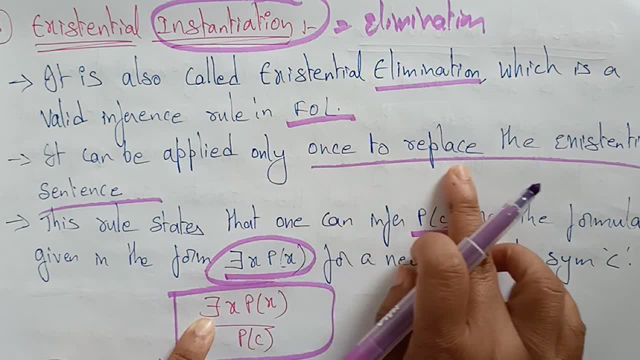 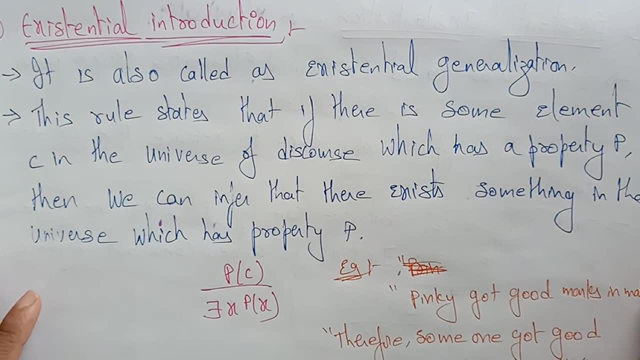 we are using there exist and it can be applied only once to replace the existential sentence. Now coming to the fourth type, that is, existential introduction, It is also called as existential generalization. So, just like a universal generalization, the existential generalization.